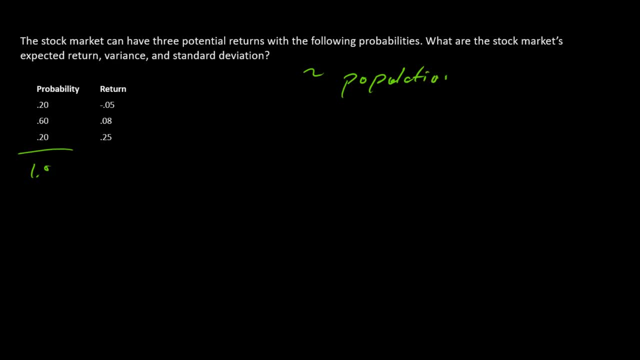 a population. We're not dealing with a sample. Okay, And so our expected return variance and standard deviation calculations are going to be exact as opposed to estimates, and they're going to deal with the probabilities and these different potential outcomes. Alright, So let's calculate expected return variance and standard deviation. The first one we have. 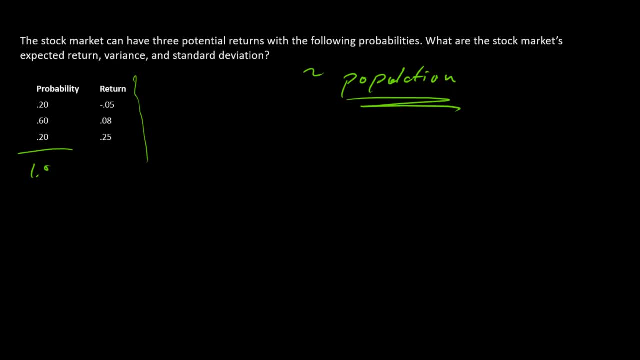 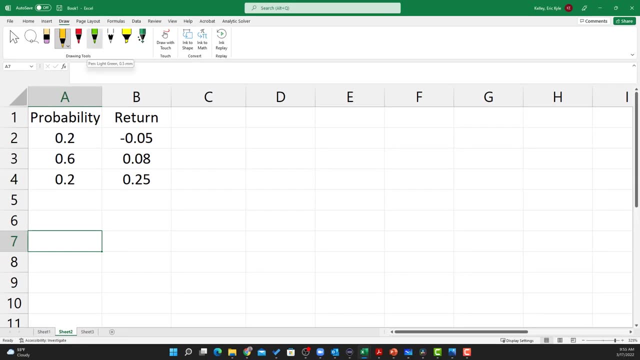 to calculate is expected return, because we're going to be dealing with a population And going to use that in the variance and standard deviation calculation. So here I've got the probabilities and returns, And so to calculate the expected return we're just going to do a. 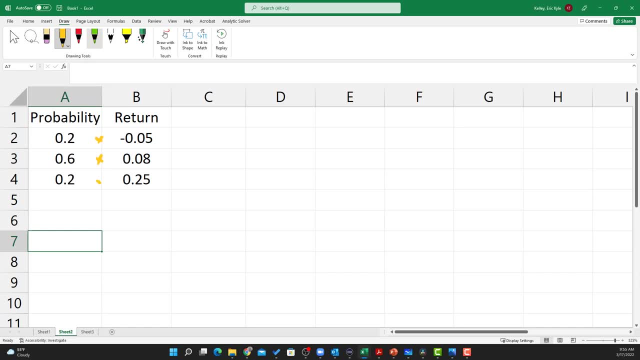 weighted average, where we multiply each probability by its return and then add them up. And so in this column over here I'm just going to call this the probability times, the return, or p times r, And so I'll just go line by line and multiply, Copy this down, So I've got probability times. 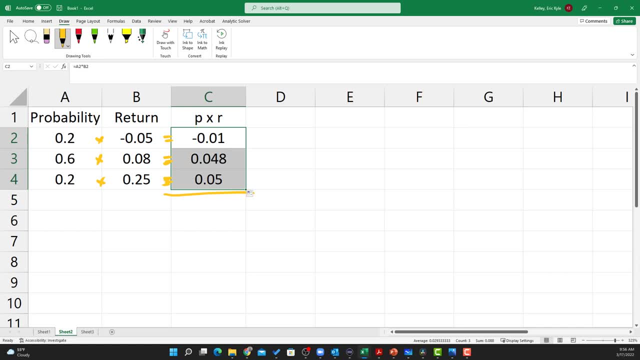 returns. And so now here we will sum these up into this cell here. equals the sum of each of these three probabilities times returns, And so that's our expected return. right there, Now let's move to the variance calculation. So the variance is going to be based on squared. 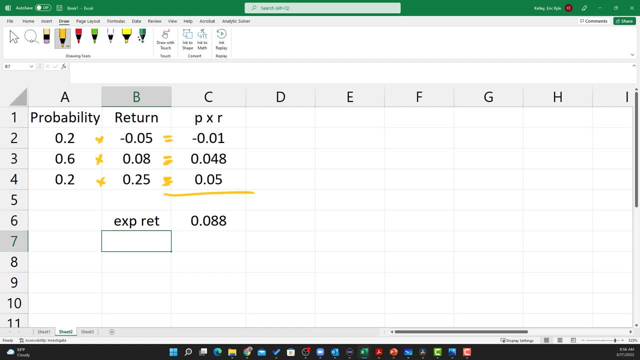 deviations from the mean. And so, again, the mean is the same thing as the expected return. So the mean is just going to be that cell right there, So 8.8%. And so let's calculate the deviation. So what's the deviation going to be? The deviation is going to be this: 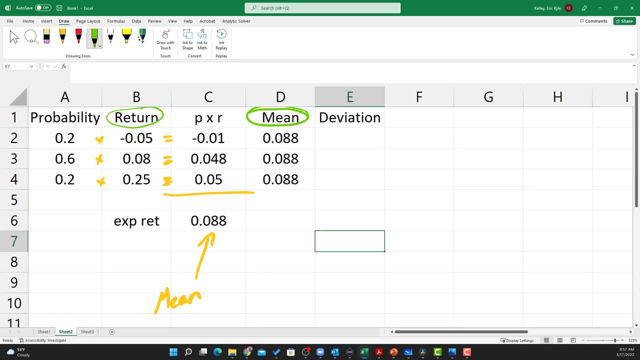 number minus the mean. So the return minus the mean, and that's going to get us the deviation Here. I have equals, the return minus the mean, And copy that down for each one of these states of the world. Now the variance is based on the squared deviation.